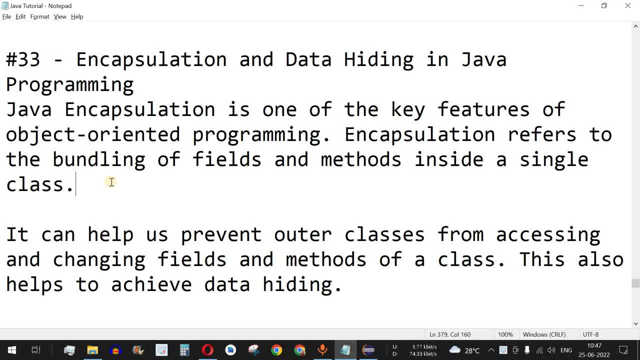 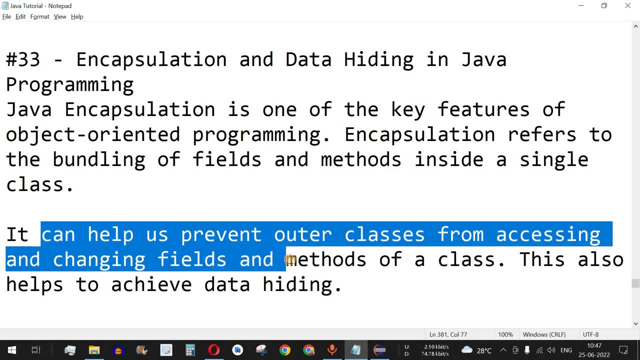 is called java encapsulation, that is, in order to encapsulate similar fields and methods inside a single class and then we can access that class to create objects in order to access those fields and methods. now it can help us prevent outer classes from accessing and changing fields and methods of 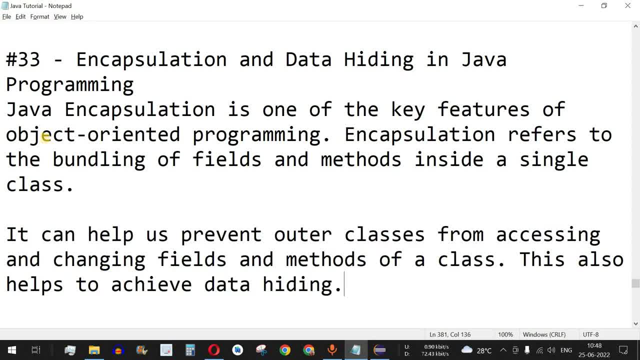 a class. this also helps to achieve data hiding. so, guys, we have two things to learn over here here. the very first thing is we will revise java encapsulation and then, secondly, we will see how we can hide the data from other classes if we don't want them to access the data directly of 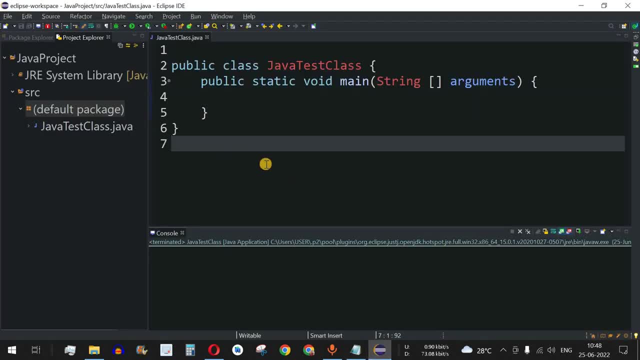 a particular class. so, guys, let us move to the ide over here now. let us say we have a class, so let's say we have class animal over here, because that's one of my favorite classes over here. we will have a string, so let's say string the name. and then let's say we have another variable, which is in: 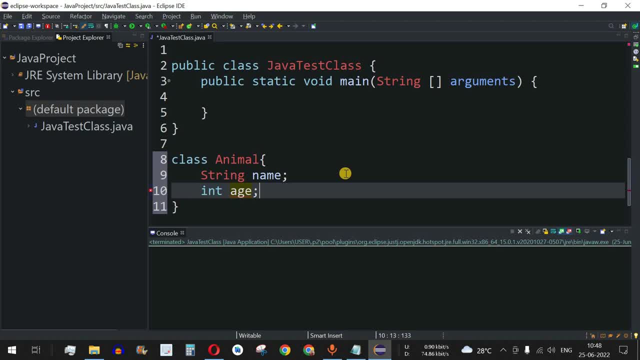 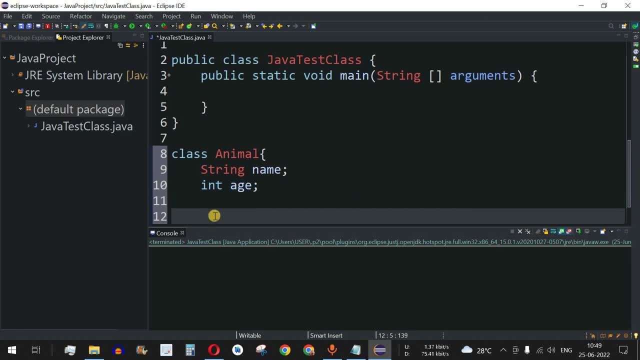 age, so it is the age of the animal that we are going to define. and then, guys, let us say we have setters and getters over here in order to access these variables. so what i can do is i can right click over here and we can go to this source option and then you can see over here: generate. 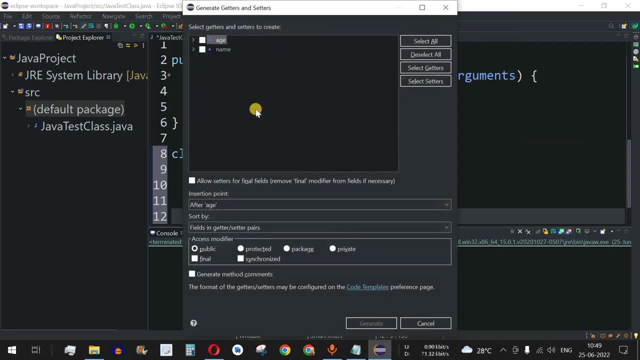 getters and setters. so i'll just click over here. so what this will do is it will ask for which variable names we want to generate the getters and setters. so over here we will select both of these variables, that is, age and age of the animal, and then we will define the age of the animal. 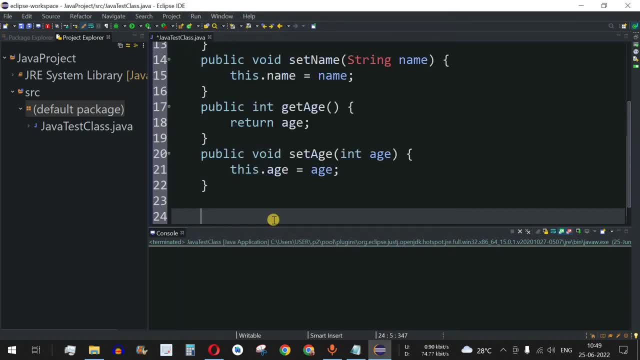 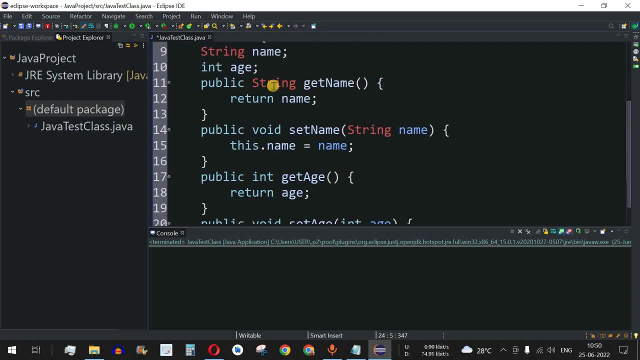 and name, and then i'll just click on this generate. so when we click on this generate, as you can see, there are certain methods that are being created over here. so the very first method is get name. so it is getting the name and it is providing us a string as the return type. so it is just. 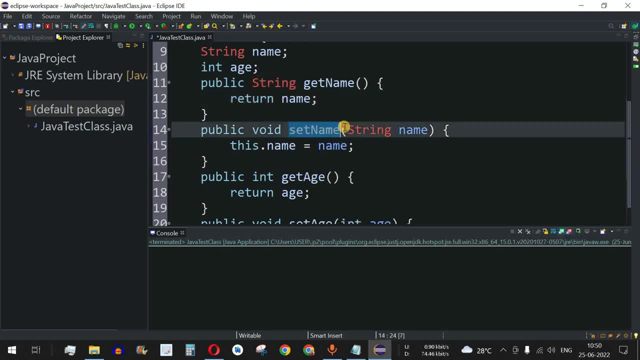 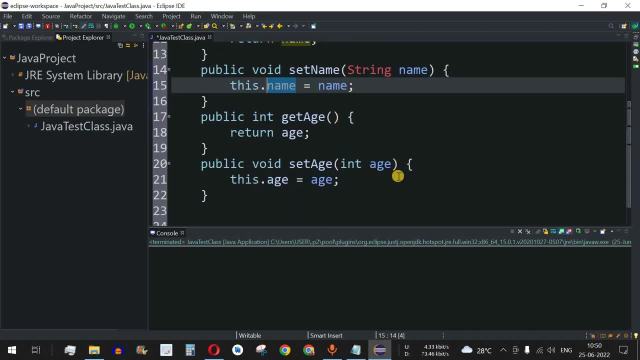 returning the name of the animal. the next method is set name, which is taking a string that is name and it is just setting this name variable inside this class and the other two methods we have similarly implemented for the age as well, that is, get age and set name and then we will just 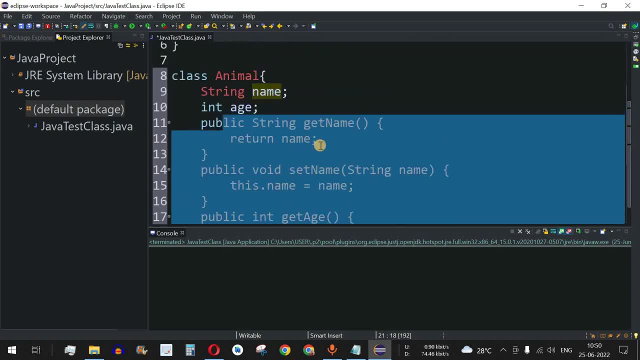 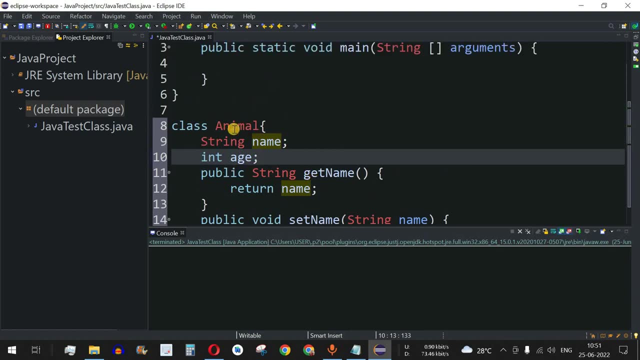 set age. so, guys, these are nothing, but these are the getters and setters for the particular list of fields that we have defined over here. now, guys, what we will do is we will create an object of this class that is animal. so i'll just copy this and paste this over here, and then create the object. 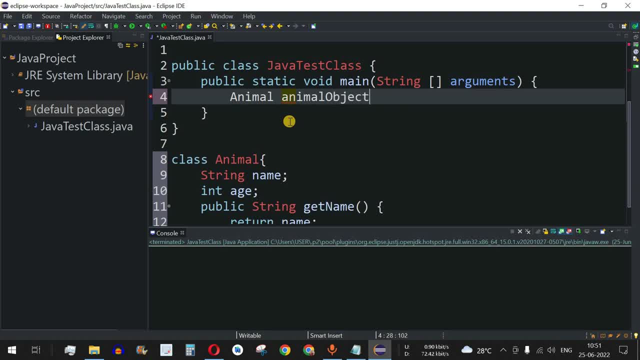 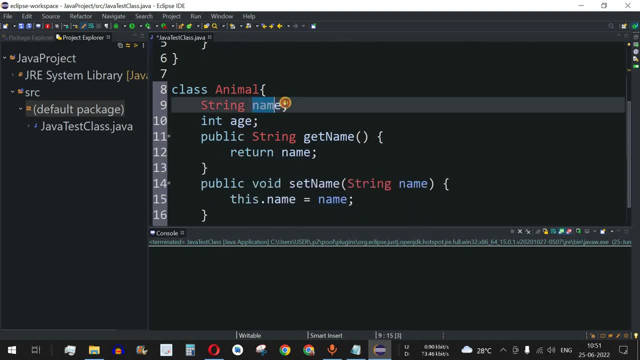 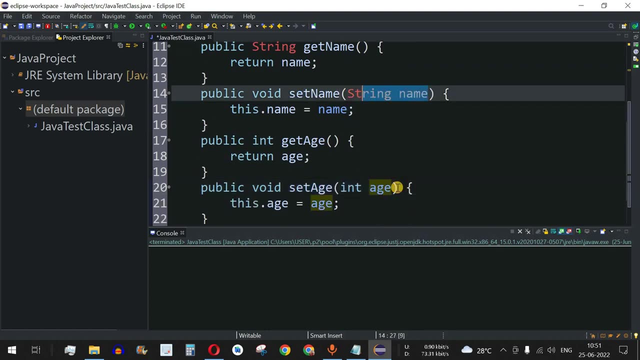 name. that is animal object. so we have animal object over here. it is equal to new animal. now, guys, we have created this object. now we can easily set the name and the age of an animal using these methods. so what we will do is we will set the name and set age. we have to provide the name and age. 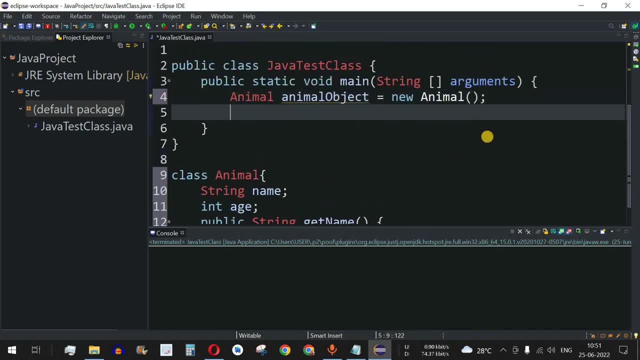 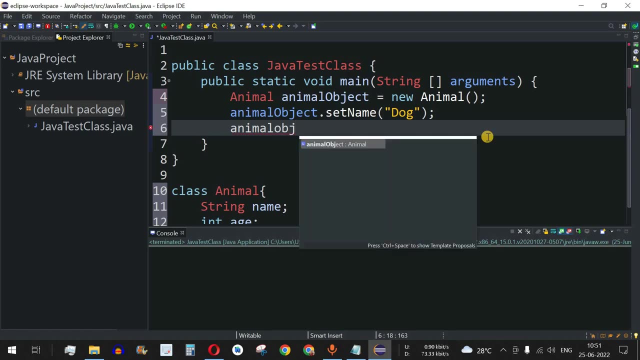 respectively in these methods. so what i will do is, the very first thing is we will set the name, so animal object, dot set name, so set name. and one of the animals is dog, so i'll just provide dog over here. and then we have animal object again in order to set the age. so we have dot set age. so 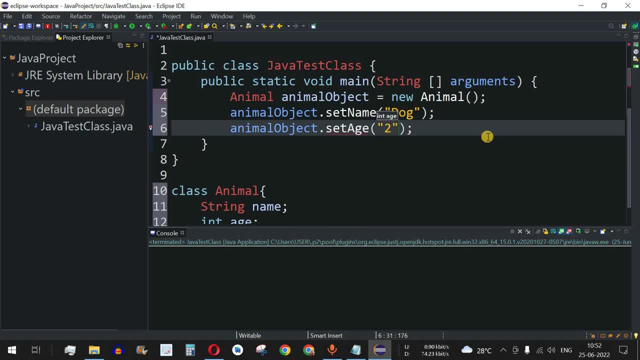 let's say the age of the dog is, let's say, two years. so i'll just provide two over here as the integer. but, guys, we have provided it inside a double quotes. so it is saying the method set age int in the type animal is not applicable for the arguments string. so i'll just remove this double quotes over. 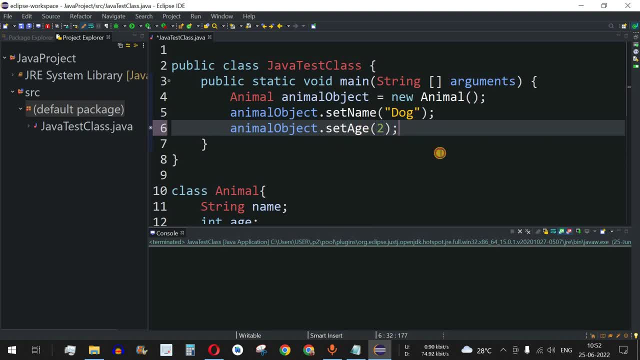 here, since it is expecting an integer. so now there is no red underline over here. now, guys, let us access these variables, that is, name and age that we have already set over here. so what we will do is we will have a print statement and inside this print statement, the very first thing is name of 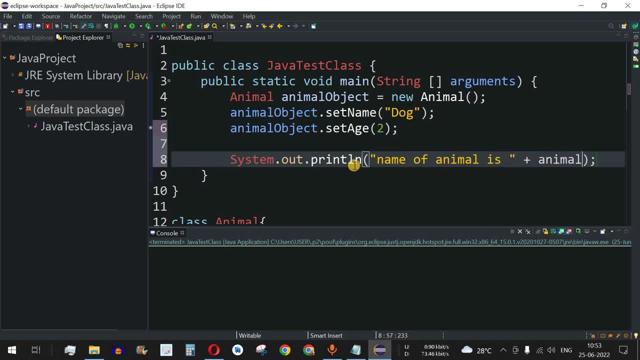 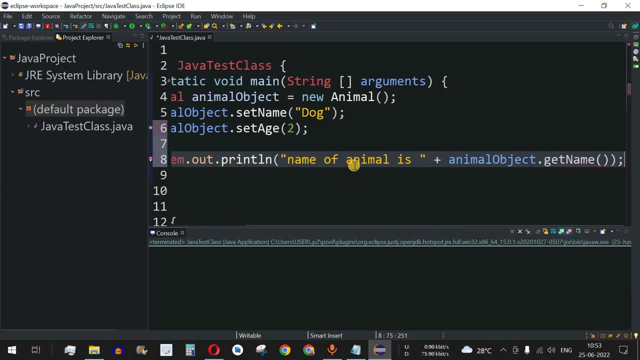 animal is, and then we will have animal object, and then we will have animal object, and then we will have animal object again, because we have the get name method. that is already implemented, so we have get name over here. so, guys, as you can see, animal object dot get name can be used in order to return. 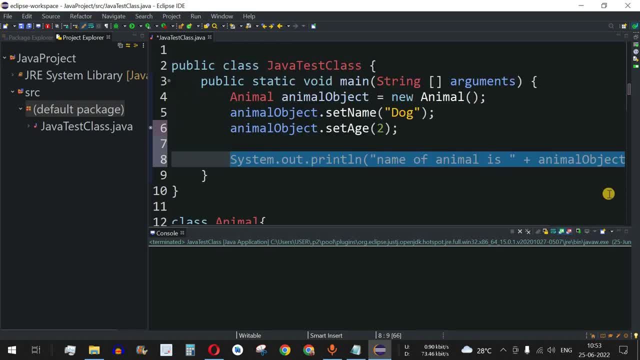 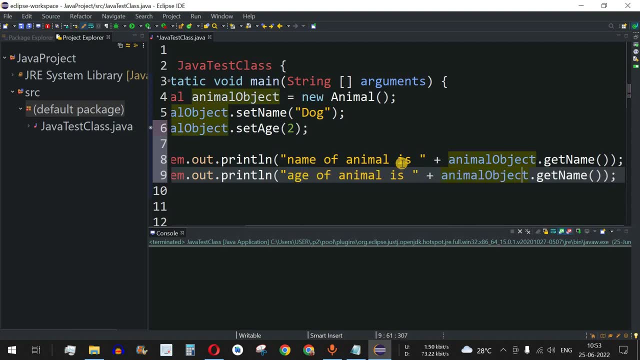 the name of the animal and then, similarly, we will return the age as well. so i'll just copy this and paste this over here and i'll just change this label to age of animal is and then we have animal object dot instead of cat name. we will have get age. so i'll just put get name and then we will have. 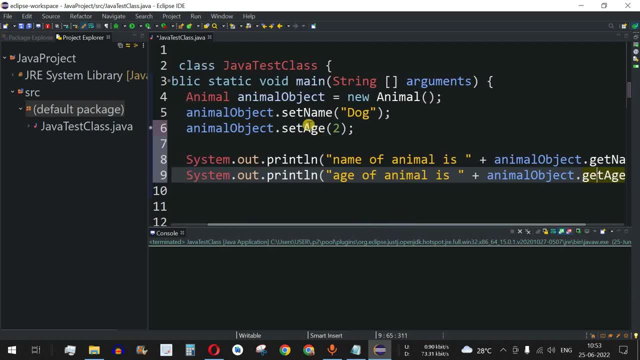 cat age over here. so, guys, in this way we are accessing all the four methods. the very first method is set name, and we are providing the name of the animal. and the second method is set age, and we are providing the age of the animal and over here we are using the get name and get age methods. 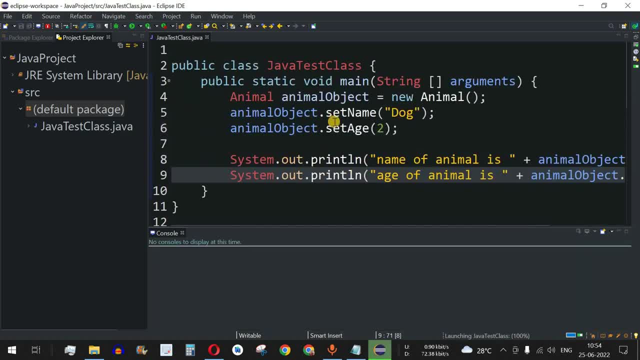 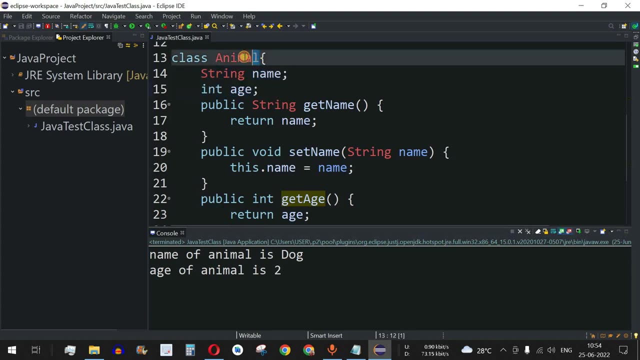 as well. now let me just save this file and try running this code now. so, as you can see, name of animal is dog and age of animal is two is getting printed over here. so, guys, in this way we have got the information by using the name and age fields of a particular class, that is, animal class. 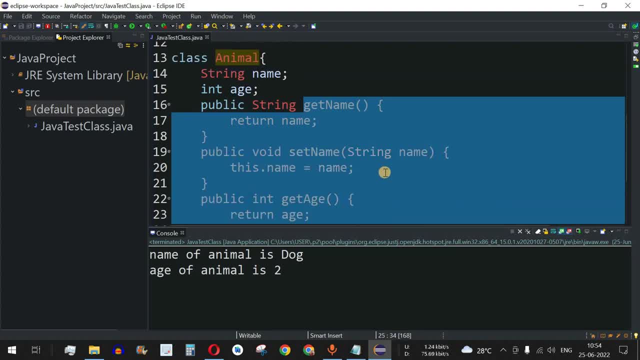 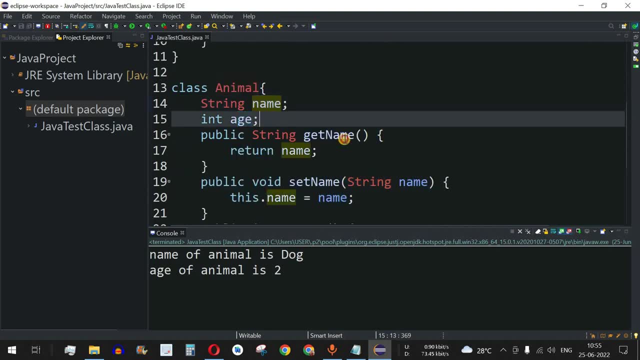 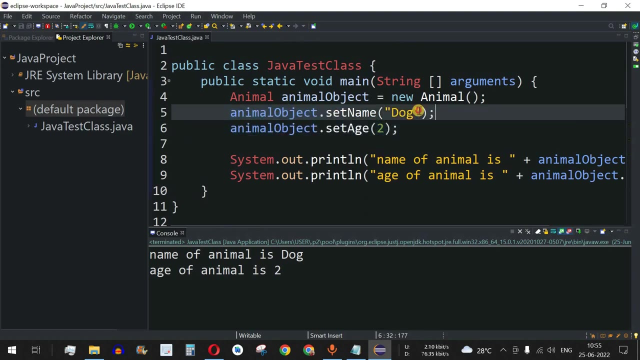 in this case, and we are using the methods in order to access them. now, guys, as far as the data hiding property of java is concerned, over here we can directly access the name and age of the animals without actually using the methods that we have created over here. so what i will do over here is: 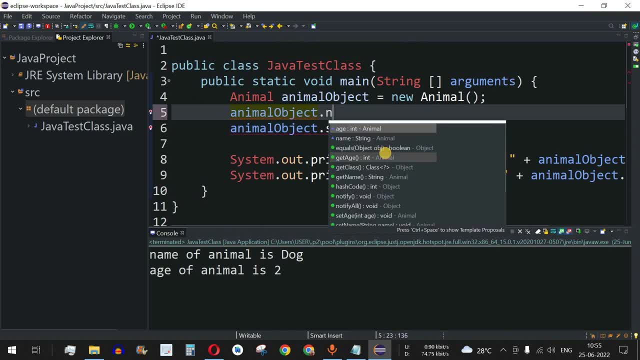 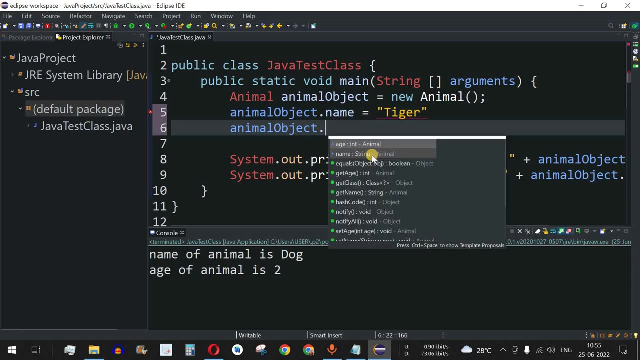 instead of using the set name, i will put dot and then name so, as you can see, this name can be accessed and we can provide equal to operator over here. and let's say we have another animal, that is tiger, and over here the age variable as well we can access easily by using the age variable. so age: 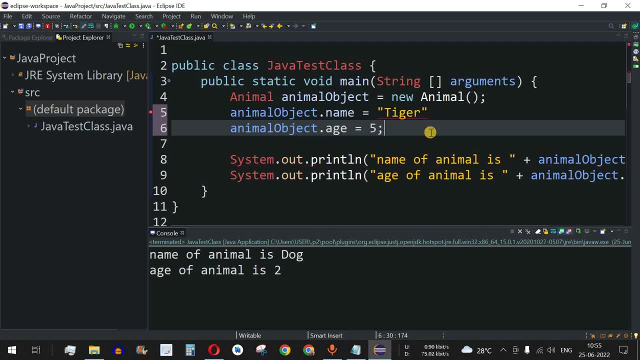 let's say it is five, so i'll just provide five over here as the age of the tiger. so we'll put semicolon over here. let me just save this file and try running this code. so, guys, one important thing over here is we are not using the set name and set age over here in order to set the name and the age. 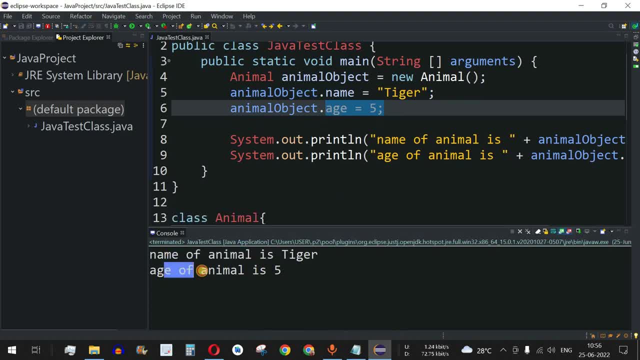 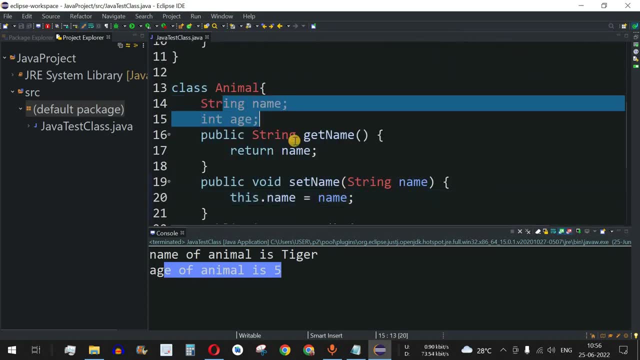 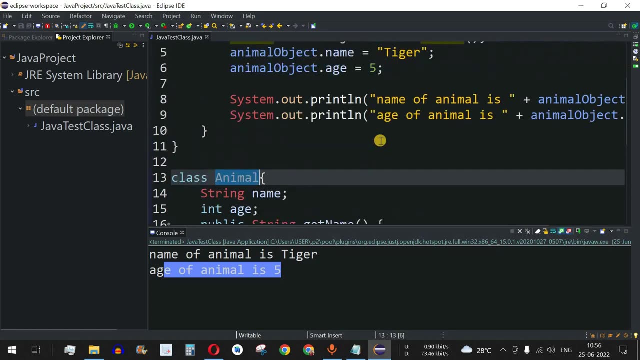 but still we can access them. that is: name of animal is tiger. age of animal is five. so, guys, though, we have achieved java encapsulation over here by enclosing these fields inside the animal class, but we have not achieved data hiding. that's because these variables of this class animal can. 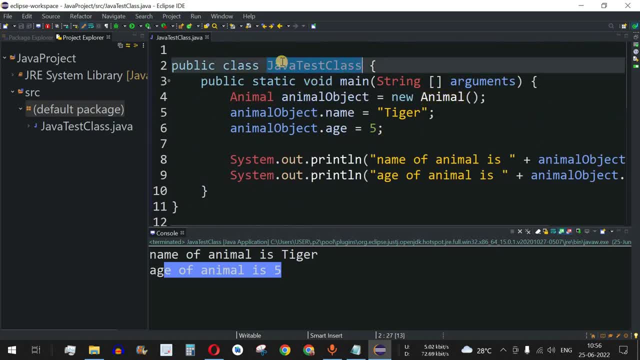 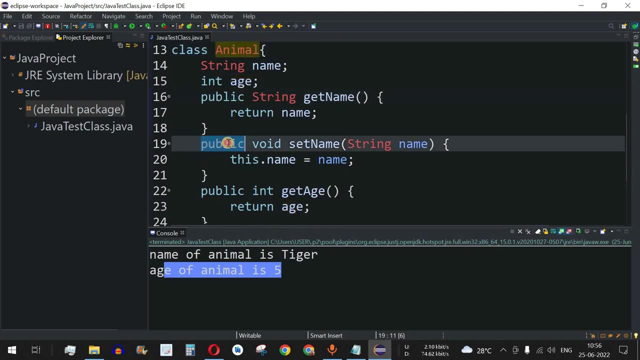 easily be accessed using the other classes. in this case, we are using java test class in order to access these variables over here. now what if we don't want them to directly access these variables? access them via the methods that are provided inside this animal class as public method. so what? 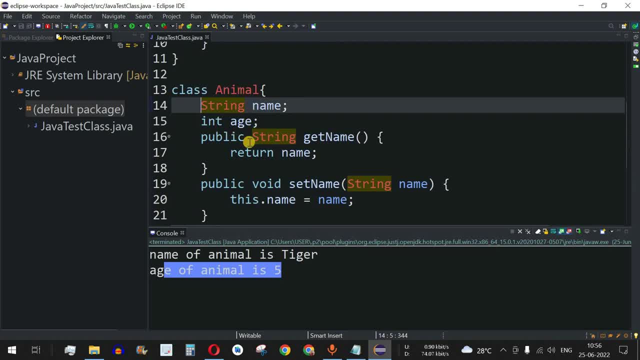 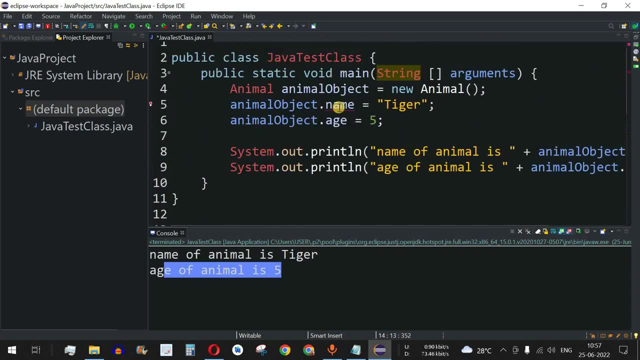 we have to do is we have to make these variables over here as private. so when we provide private keyword over here before the string variable and we scroll over here on top, as you can see, there is a red underline- that's because we cannot directly access that particular variable now. 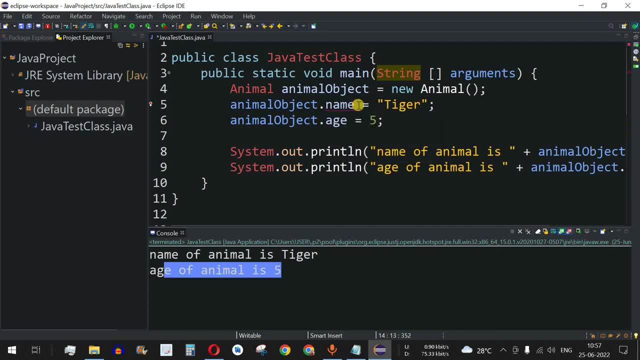 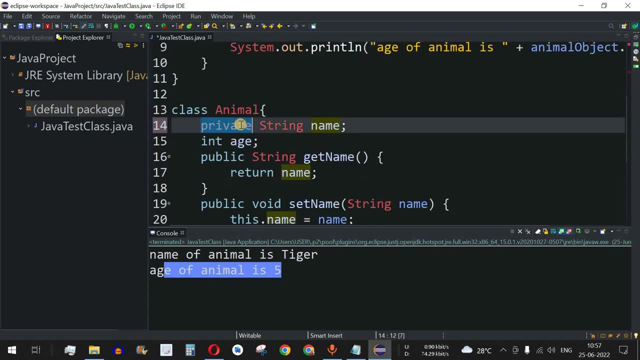 it says the field animal dot name is not visible. that's because we have made it private. the age is still visible because we have not made it private. so we have to make it private. so we have to make it private yet. so i'll just copy this private keyword and paste this over here for the age. 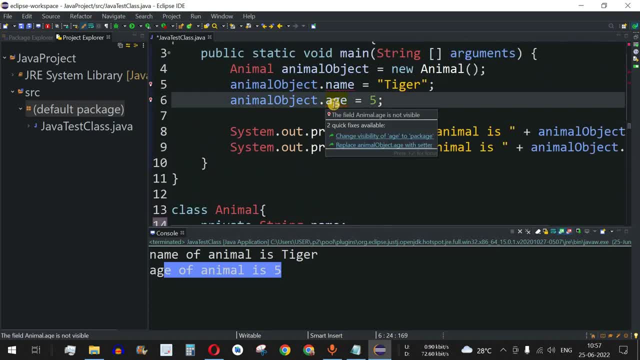 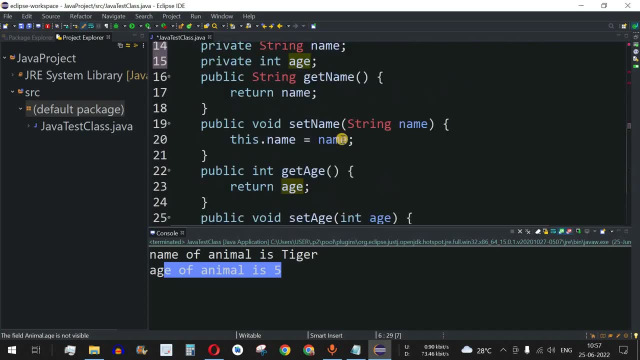 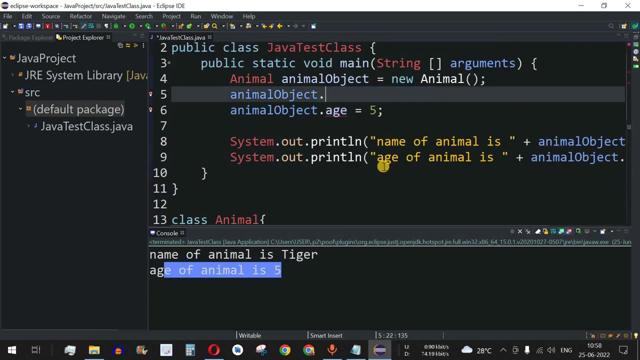 variable as well, and over here for age as well. we cannot access them directly, so now the only way in order to access these names and age is through the methods that we had seen previously, using the set name and the set age methods. so what we will do over here is we will remove this name and we will 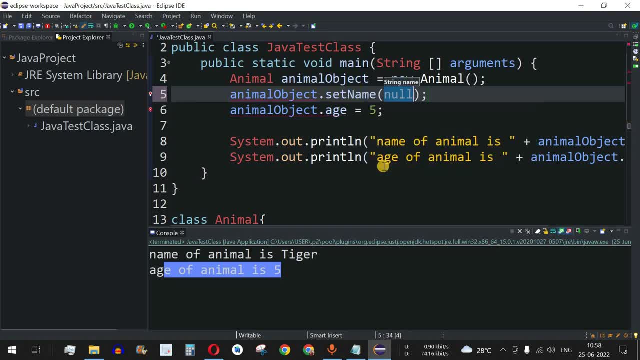 again call the set name over here. so we have set name. so again we will put the name of the animal as tiger and let's say: we'll remove this age and we will provide set age method. so we have set age. and then let's say the age of the tiger is seven years, so i'll just provide seven over here. so now there. 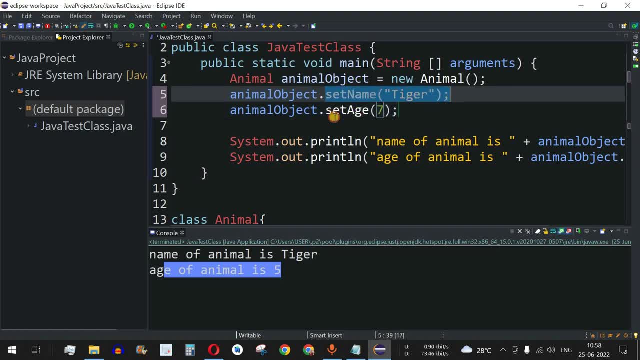 is no red underline, that's because we are accessing the public methods of that particular class. so let me just save this file and running this code now. so, as we can see, name of animal is tiger. that is what we had said, and age of animal is seven. so that is what we had said over here in the set age. 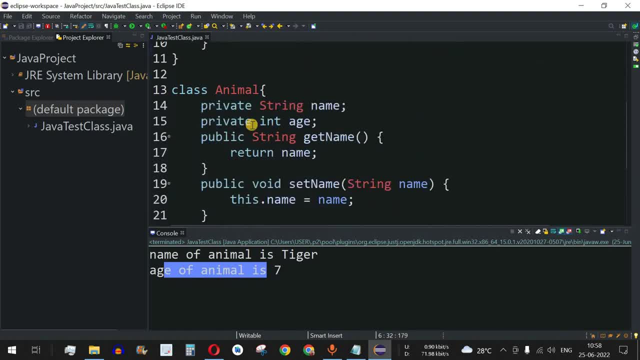 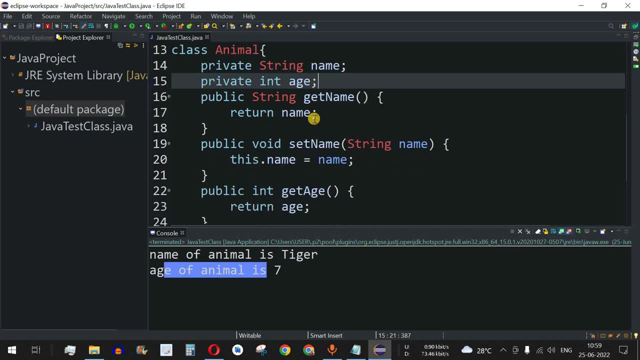 method and, guys, if you have any questions, please feel free to comment in the comment box below. and this way, we can also achieve data hiding property of the java using this access modifier of private keyword. so, guys, hopefully you have got enough knowledge about java, encapsulation and data. 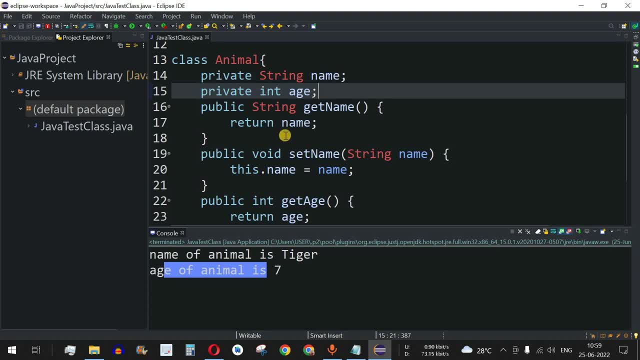 hiding and how these can be achieved using the access modifiers. so, guys, that's it in this video. please make sure that you like this video so that it reaches to more people, and subscribe to the channel so that you get the notifications on upcoming videos as well. the next video that we 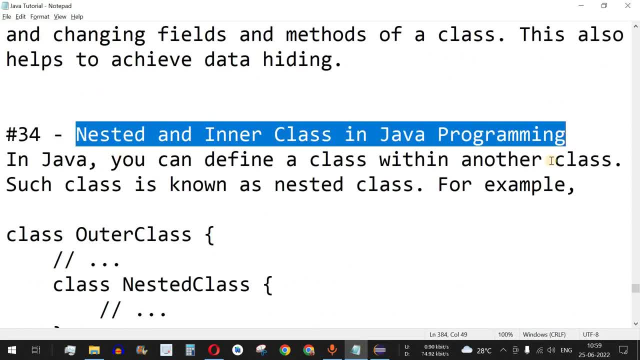 are going to talk about is nested and inner class in java programming, so stay tuned. 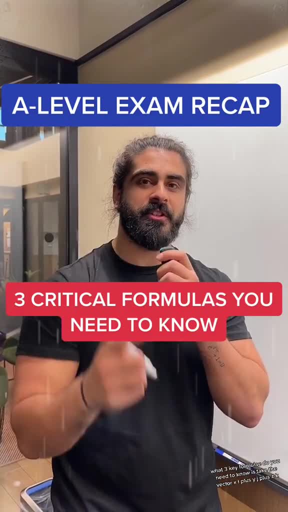 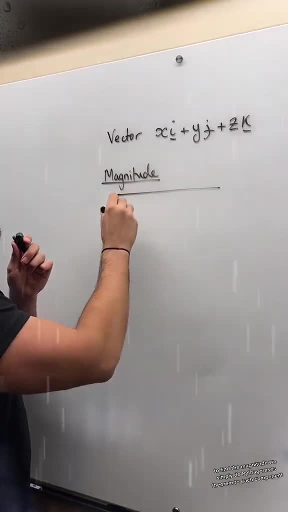 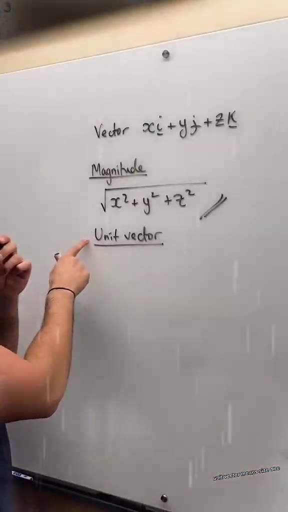 A-level vectors. What three key formulas do you need to know? Let's take the vector xi plus yj plus zk To find the magnitude. we simply do Pythagoras' theorem to each component. Next one is a unit vector. Unit vector means size 1..